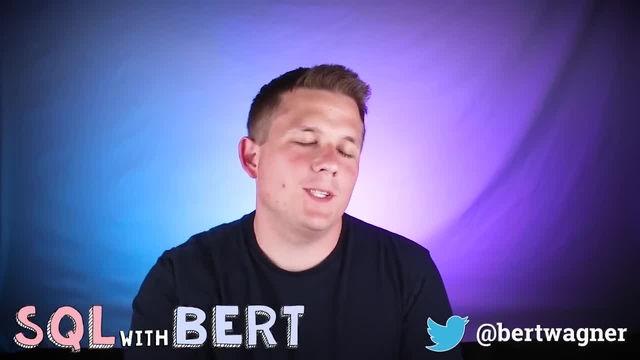 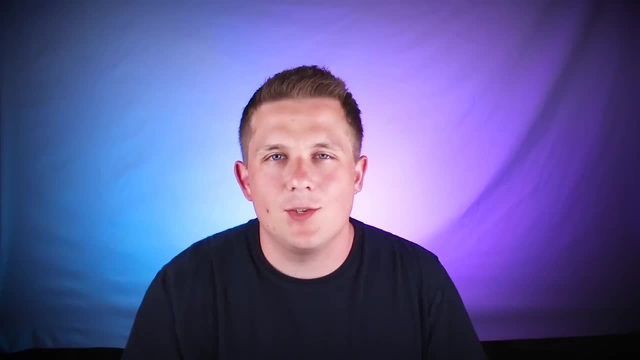 Welcome back everyone and thanks for joining me again this week. First off, before I get into the video, I just want to thank you guys because after last week's video I passed the 2,000 subscriber mark, which is something I wouldn't be able to do without you. So thank you very much for subscribing. I really appreciate it and I'm glad to hear all your comments and feedback. right that these videos are helping you. That's been my goal and it just makes me really happy to hear that. 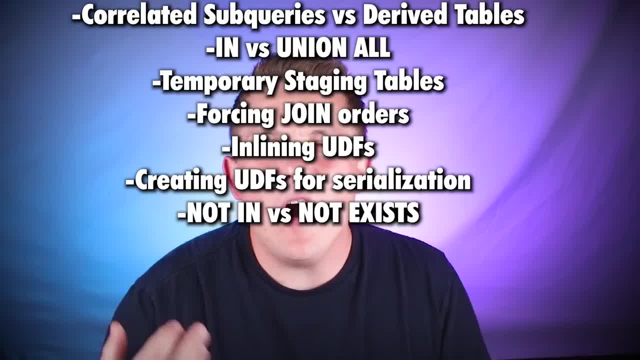 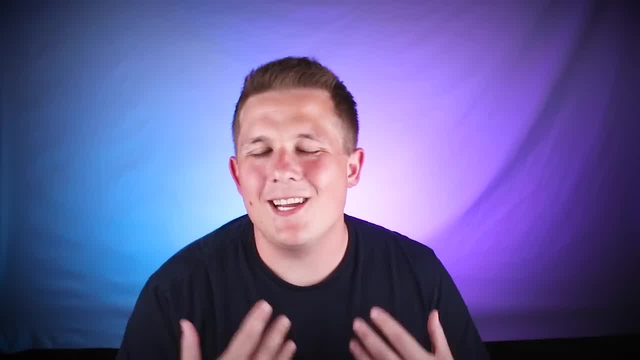 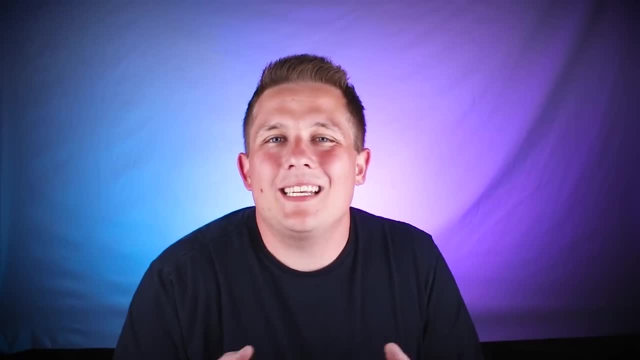 And so today we're going to have a rapid fire video for all the different techniques that you can use to rewrite a query to improve performance. This topic is very near and dear to my heart because for a long time, when I started writing SQL queries, I often ran into the situation of needing to rewrite a query for performance. 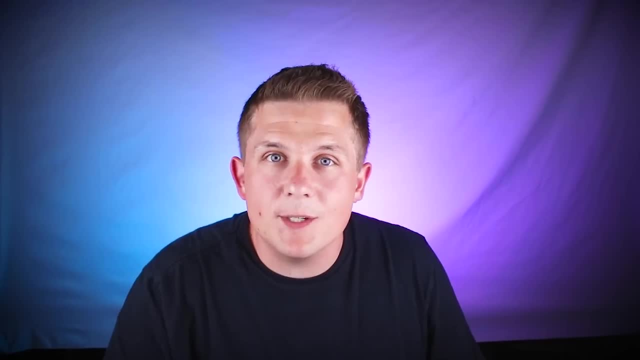 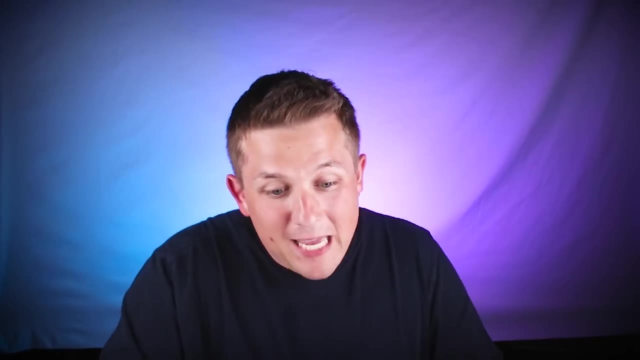 I couldn't always do things like add indexes or change server settings because I would have a lot of restrictions around the database that would prevent me from doing that. Things like vendors databases where you can't touch anything, or size restrictions, right like maybe there's just not enough disk space. 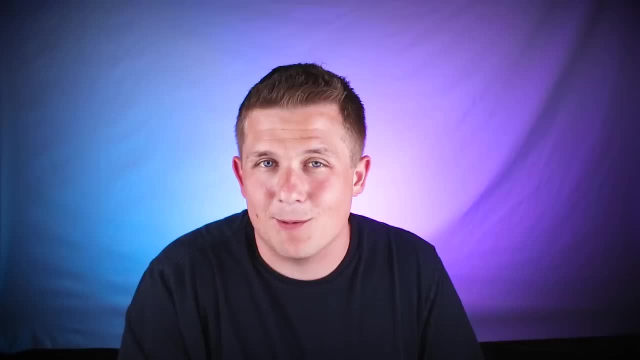 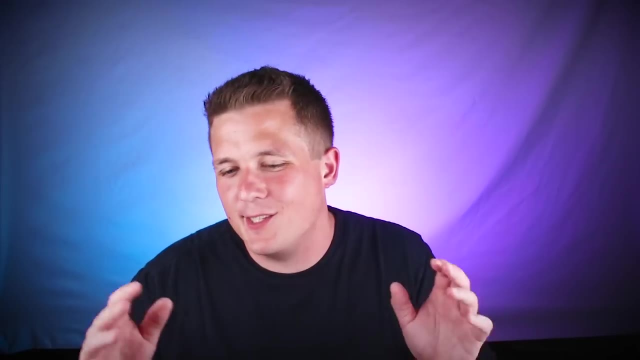 And I couldn't get more disk space allocated in a timely manner, right to be able to add more indexes or things like that, And so I learned a lot of these techniques over time, from conference presentations to blog posts to just talking to people about how they rewrite their queries. 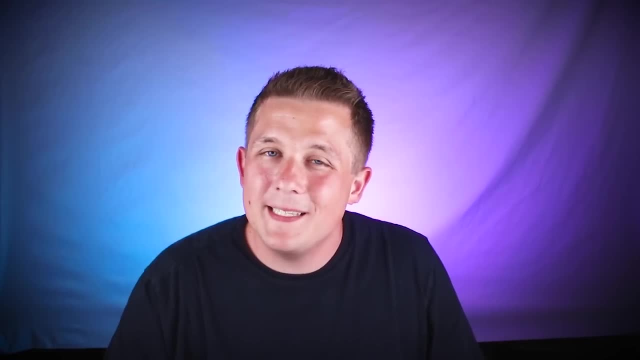 And while I feel pretty comfortable using all these now, when I was starting out, I really wish there was a resource that kind of listed all these or went over all these different topics to just help me generate ideas of how I can refactor a query for better performance. 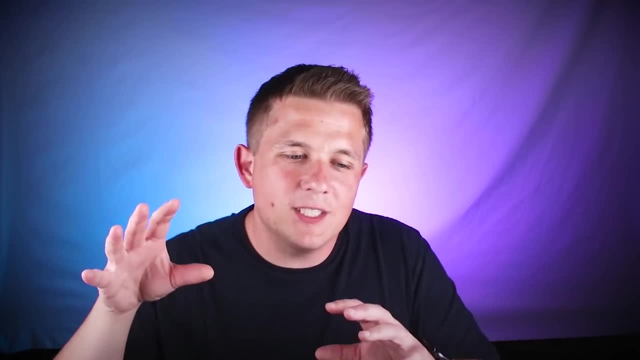 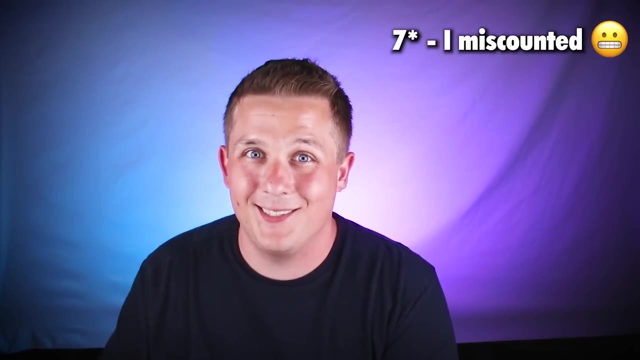 And so, with today's video, I'm going to try to do that. We're going to take a quick look at the videos- the past four videos in this series- as well as discuss eight other techniques you can use for refactoring a query in order to improve performance. 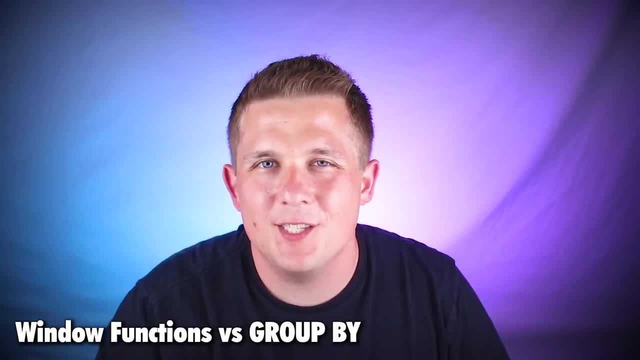 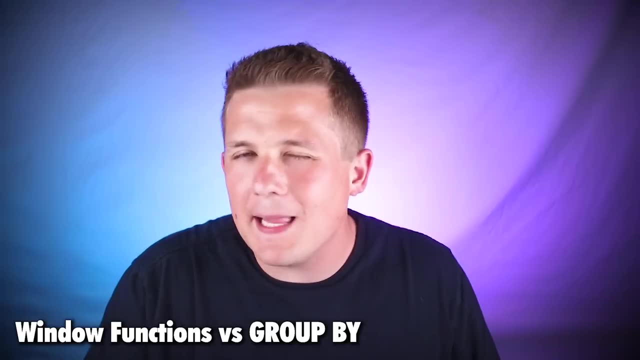 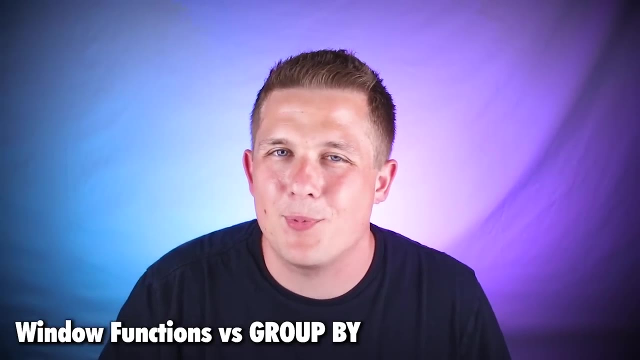 So in the first video of this series we looked at window functions compared to writing queries using group by statements. I love window functions but sometimes their performance can be a little lacking because of their use of tempdb And the fact that a lot of times they will block your query execution right, preventing from the execution from continuing on until one specific part has completed. 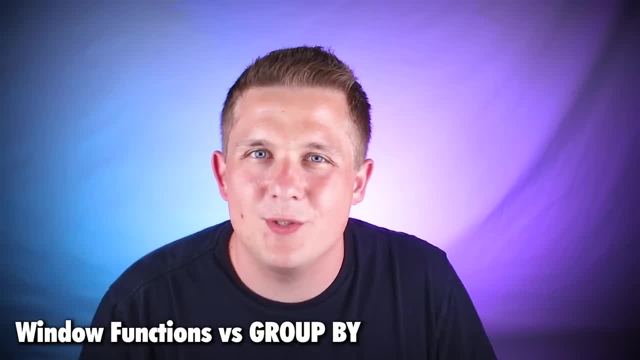 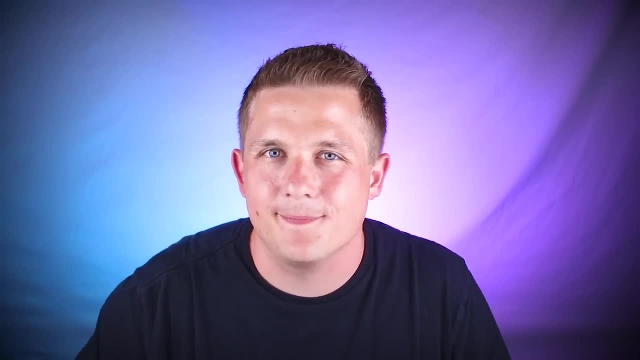 So the remedy in that case is just to rewrite your window functions using the good old fashioned group by and sub queries to get the same result that you would with the window function. In the second video we looked at correlated sub queries Versus derived table queries. 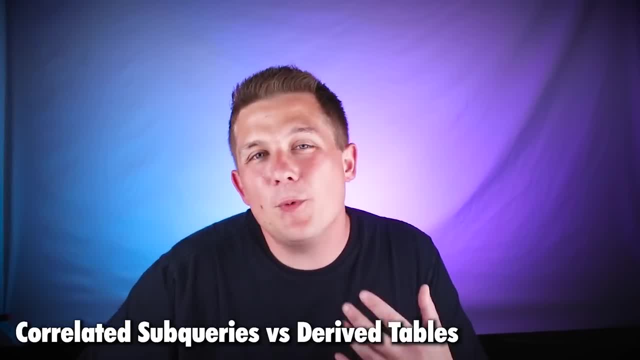 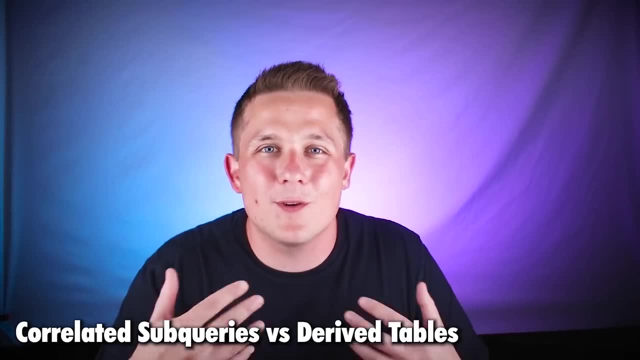 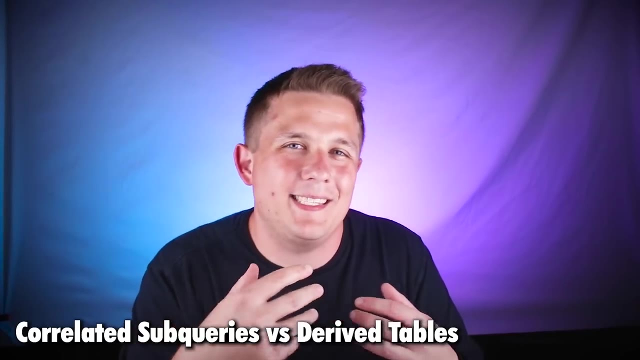 Restructuring your query logic from the former to the latter can really improve performance in a lot of situations, because correlated sub queries will often have to re-execute query logic over and over again. It basically becomes kind of like a cursor right versus using a derived table query will act more like a set based query operation, which will improve performance. 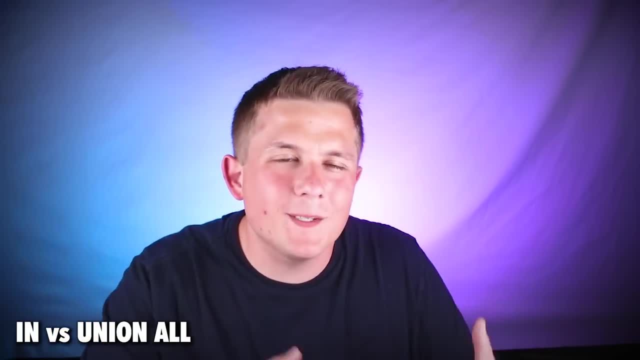 Another technique we looked at was rewriting our queries with ORs or INs to use union ORs. Another technique we looked at was rewriting our queries with ORs or INs to use union ORs or INs to use union ORs or INs. to use union ORs or INs. 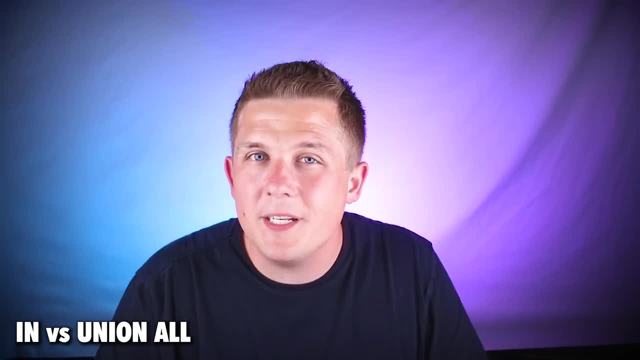 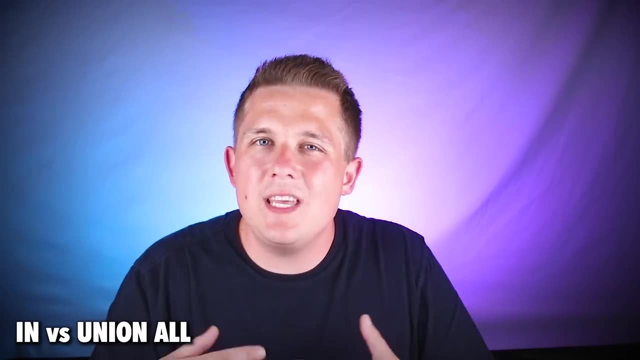 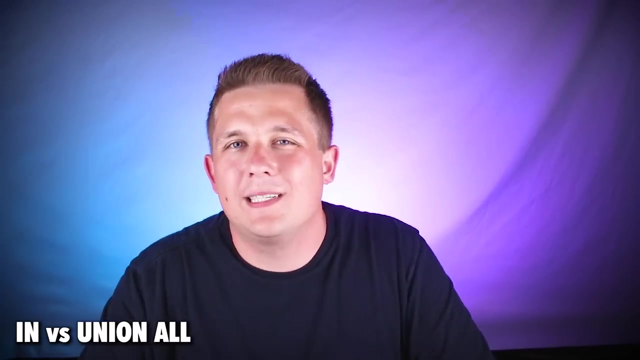 Instead, in cases where our data is not evenly distributed or in cases where we don't have covering indexes for our data, switching from an IN to a union OR could actually improve query performance, because it'll force SQL Server to kind of look at each different value that we're filtering on on its own and decide what's the best way to filter out that data from our table. 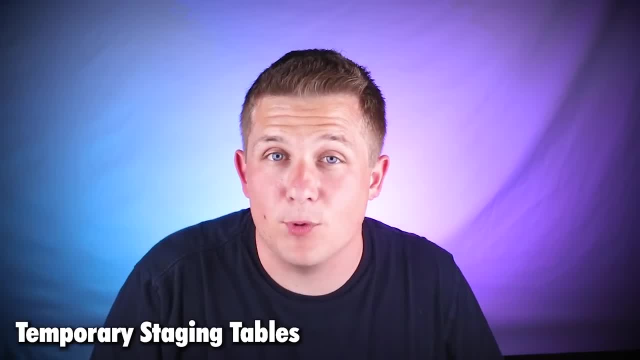 Finally, I had a video on using temporary staging tables right taking a long query or a query that is using a lot of tempdb. Finally, I had a video on using temporary staging tables right taking a long query or a query that is using a lot of tempdb. 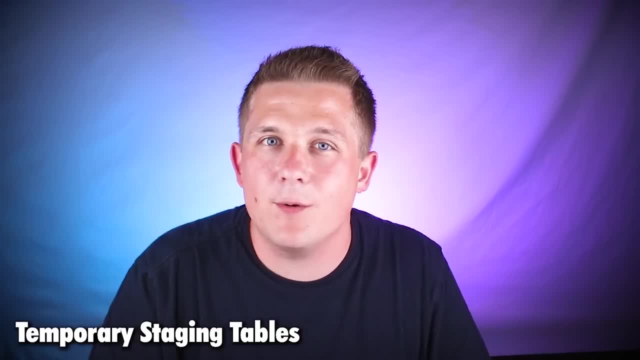 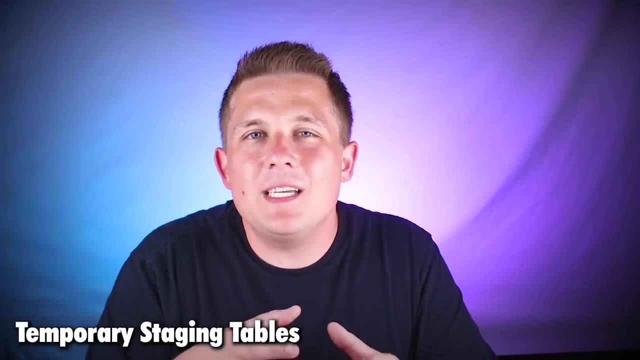 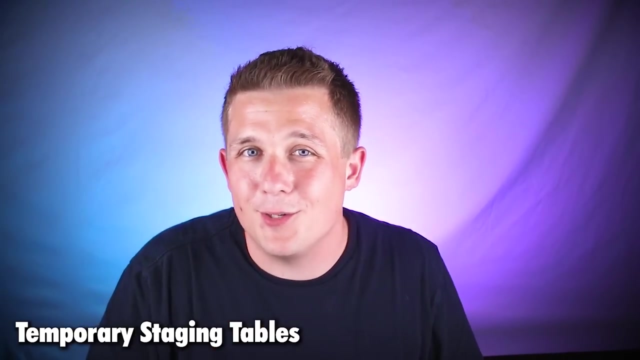 Finally, I had a video on using temporary staging tables right, taking a long query or a query that is using a lot of tempdb And just inserting a temporary table into the flow of that query to improve performance. Not only can you reuse more of your query data that way, but you can give SQL Server better information about your data so that in return, right, the query optimizer is able to create better execution plans for you which will perform faster. 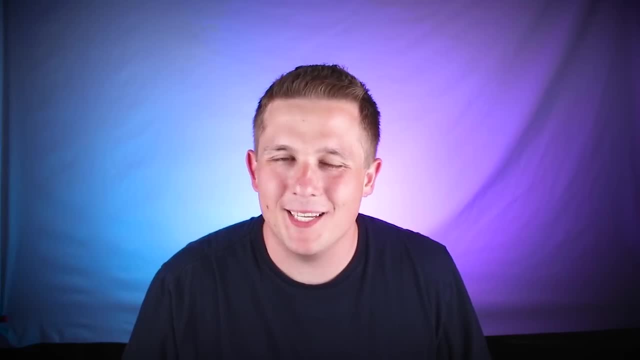 And while I created videos for those four techniques in particular because those are the ones that I find myself using the most often, And while I created videos for those four techniques in particular because those are the ones that I find myself using the most often, 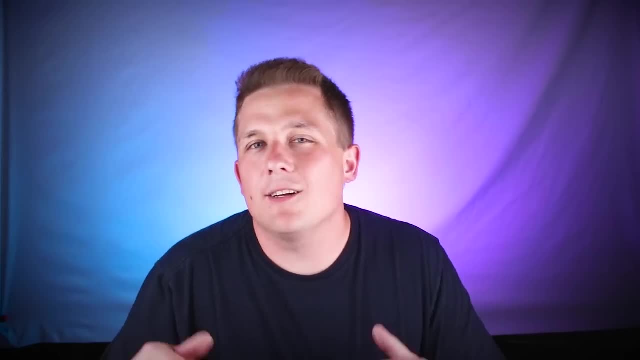 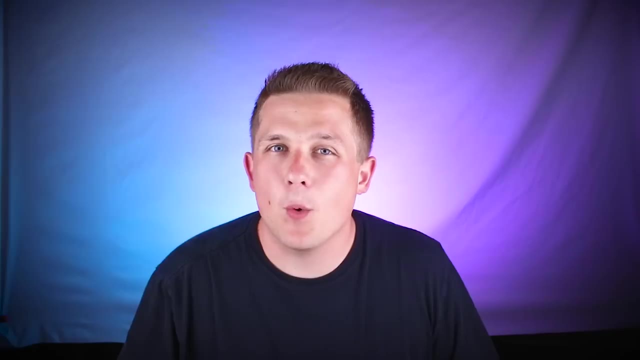 I've also added a bunch of other techniques that you can use to rewrite your own SQL queries. If you check out the blog post in the description below, you'll find that I've linked to a lot of other resources around the web that discuss these techniques. 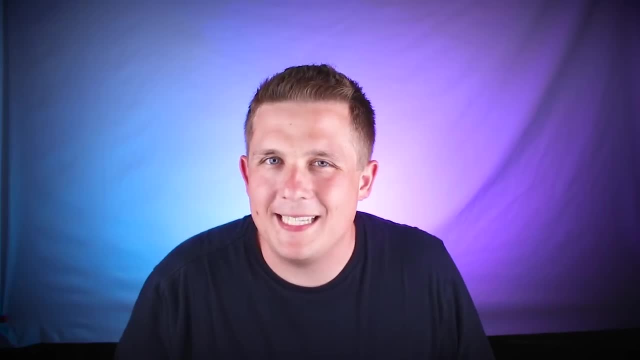 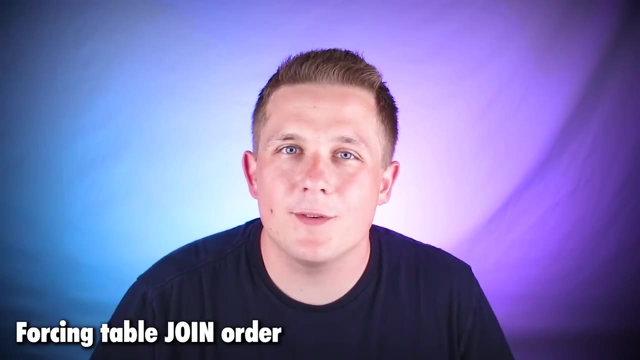 So if you want to learn more, be sure to check those out, But for now let's talk about these eight remaining techniques. So one technique you can use is forcing the join order of tables. Normally, SQL Server decides what order it wants to filter and join your data. 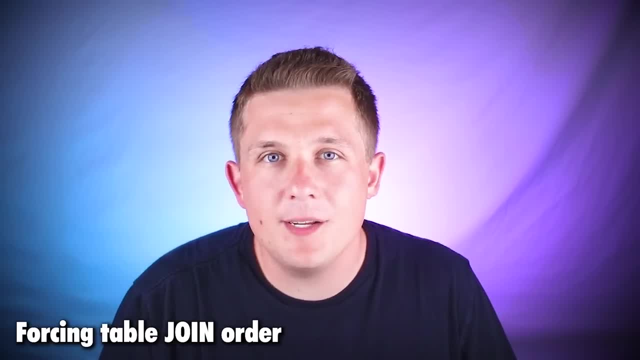 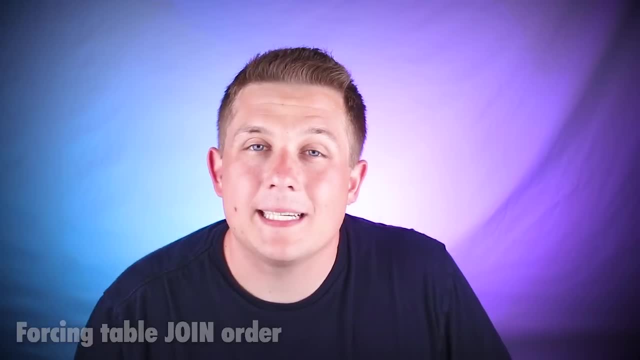 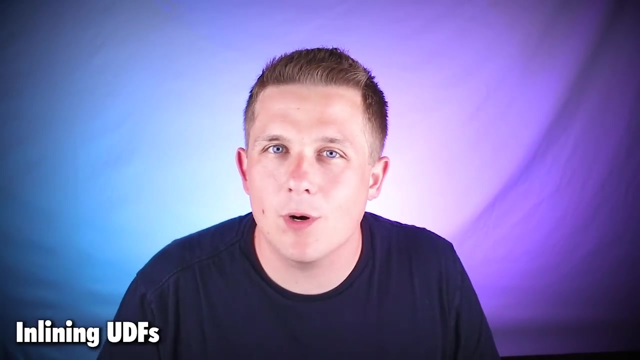 But in certain situations where it's maybe lacking good information about the correct join order or what the correct join order should be, you can force a join order by using a blocking operator like a top. Another technique you can use is to convert your UDF functions just to be directly in line as part of your SQL query. 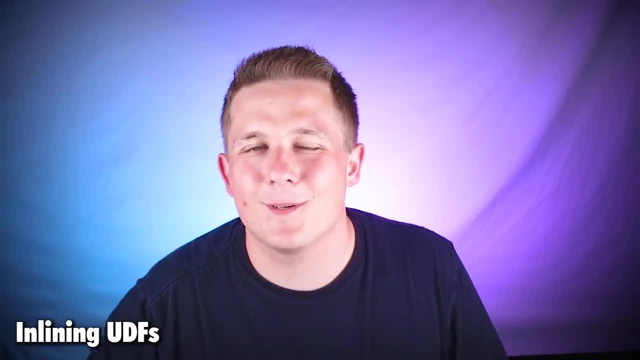 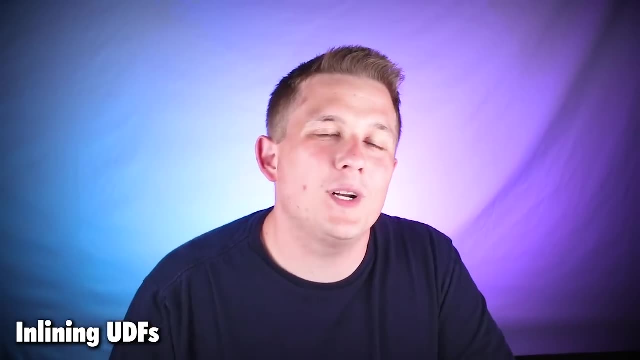 In certain situations, this will actually be fixed automatically as part of SQL Server 2019.. But until then, it's a good practice to, if you can, you know, take your logic out of a function and put it back into your query. 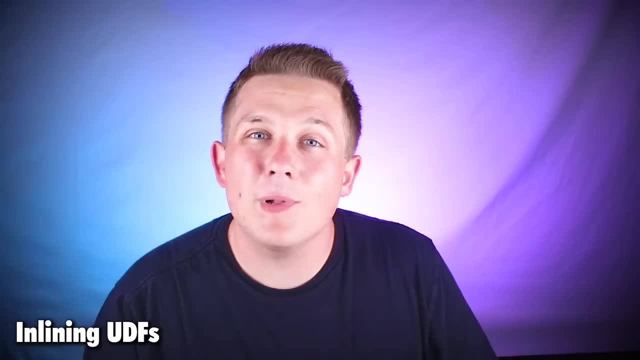 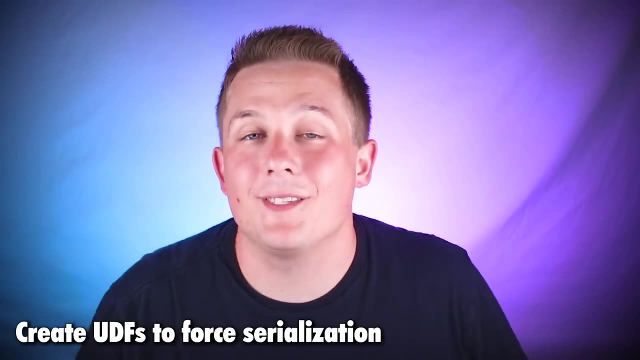 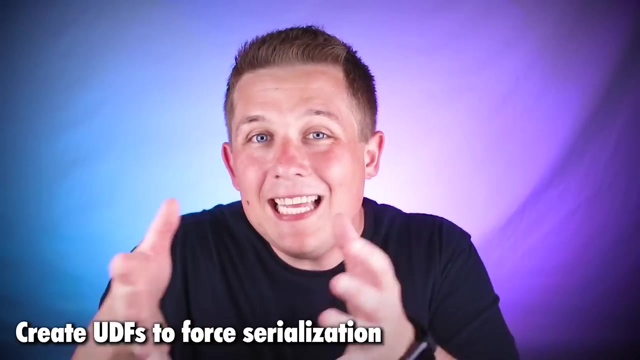 SQL Server is going to generate much better estimates, It's going to be able to use parallel plans and, overall, it could improve your query performance dramatically. On the contrary, though, sometimes you may not want your SQL Server to parallelize your queries, And in those cases it may make sense to actually put your query logic into a function, because that'll force a serial plan. 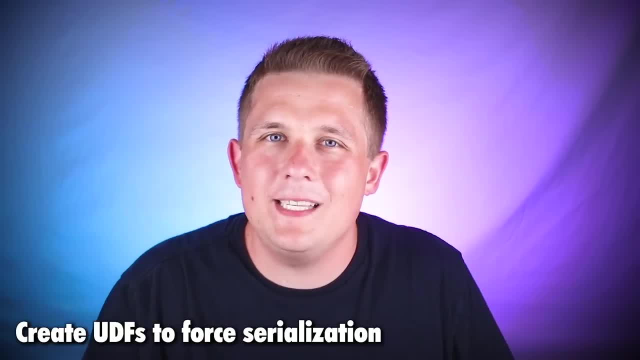 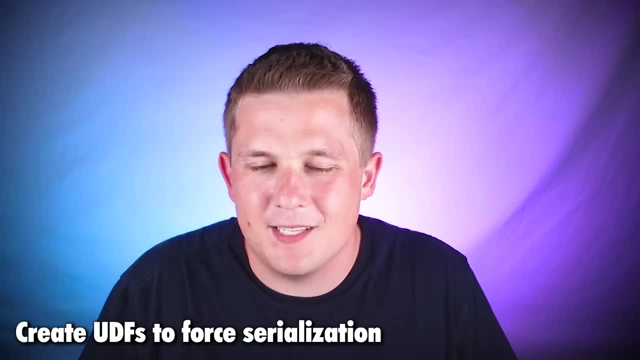 Putting your logic into a scalar function- right, if you're doing it for the right reasons- could actually generate a plan which will be more efficient, especially in those cases where parallelism, the overhead of parallelism, or maybe really skewed data that you can't change right, would benefit from a serial plan. 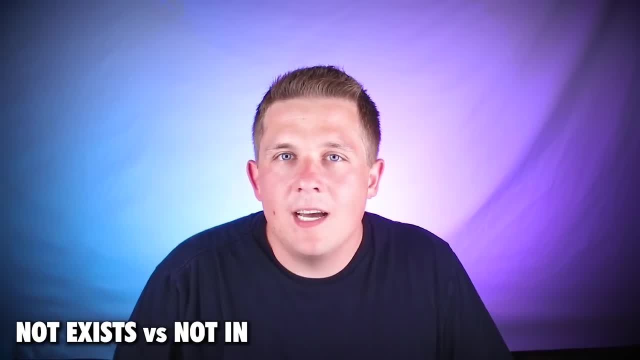 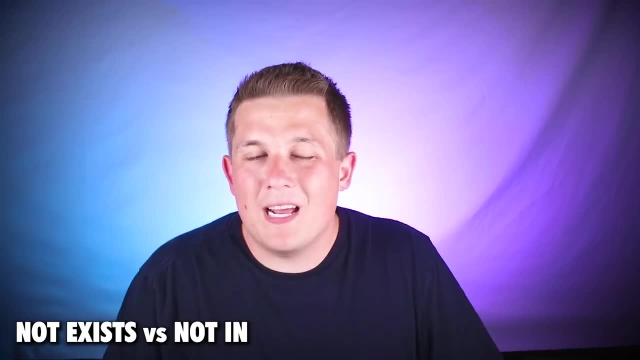 So next up is using not exists instead of not in. Generally they'll perform about the same, but under certain situations, under certain conditions, not exists will perform better. So it's always worth trying to use not exists- especially if your query is using not in- to see if you can get performance improvement there. 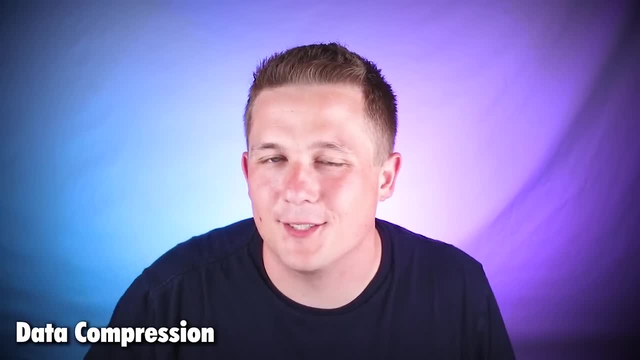 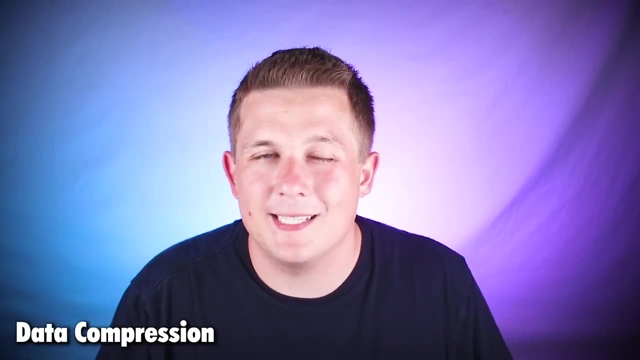 Another thing you could try to do is to add table compression or index compression. Generally, people think of data compression as, say, a storage saving measure. right, because you're compressing your data, so it's taking up less space on disk. 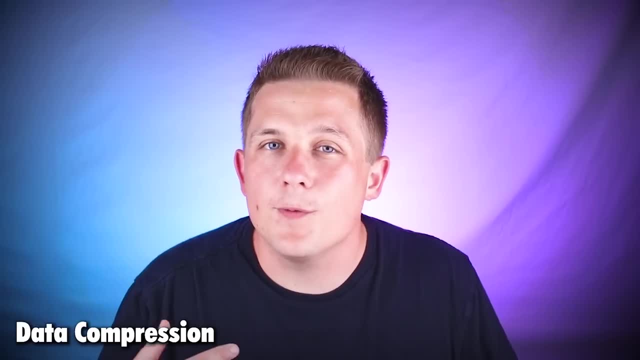 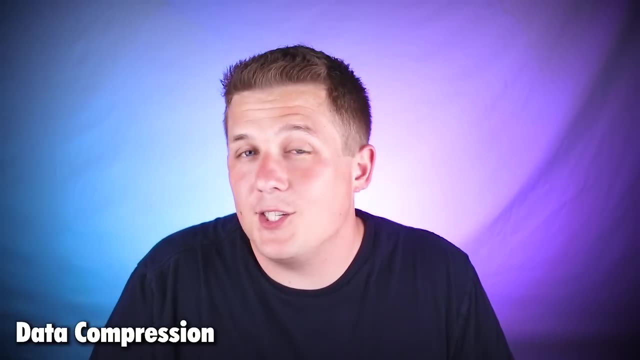 But in certain workloads, compressing your data could actually improve performance, While there is a CPU overhead to decompressing your data in SQL Server in certain situations. right, because the data is compressed, it's taking up fewer pages of data in memory. 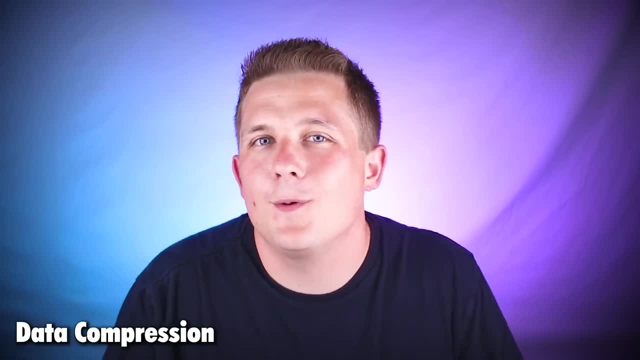 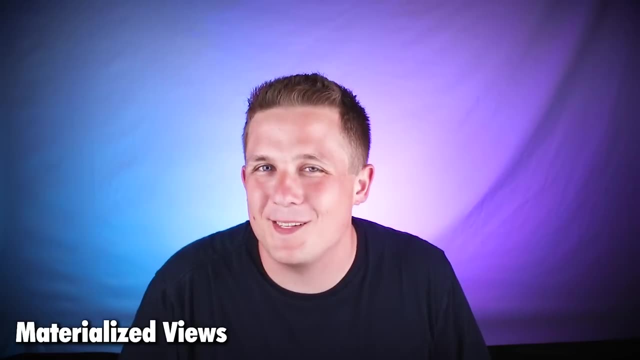 In the buffer pool. you can actually see better performance if your data is compressed. Materialized views are another option. Materialized views are another option. Materialized views are another option. This is particularly useful in vendor database environments where you can't touch the original tables. 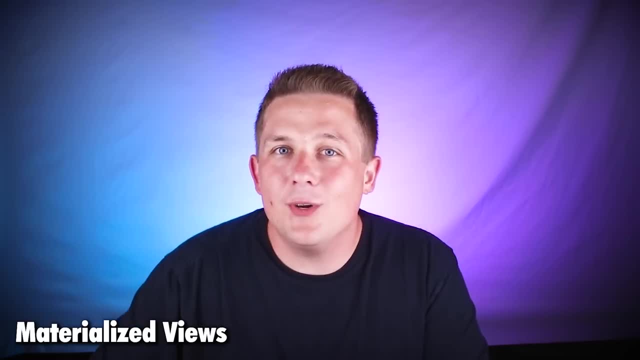 But if you can create a view and if you can index that view, you could get a lot of the same performance benefits of if you were just to index those original tables in the first place. So that's definitely one that I use a little bit more frequently than these others. 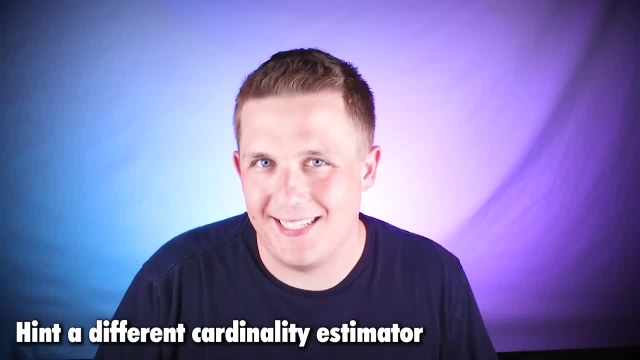 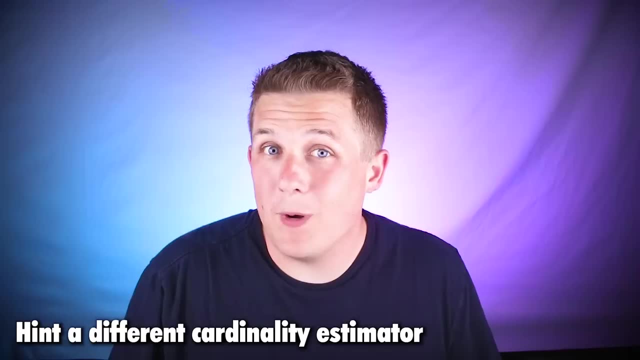 Another option you have available is to change the cardinality estimator for your query. The new cardinality estimator that was introduced in SQL Server 2014 works really well for a lot of data. for a lot of data, different queries- because the assumptions of the cardinality estimator, of how it makes 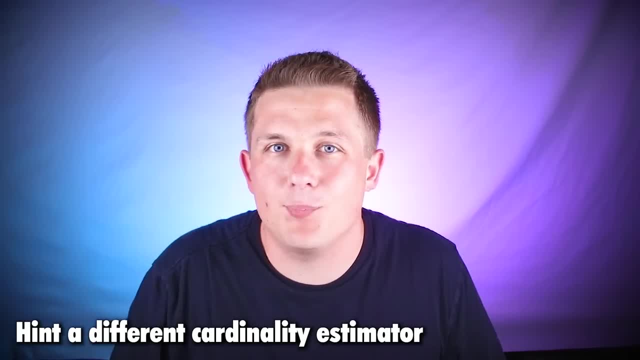 assumptions about the data have changed, but in certain situations the performance is actually worse. So one quick and easy way to just see if your query performs differently is just to switch back to the old cardinality estimator by using an option to force that legacy cardinality. 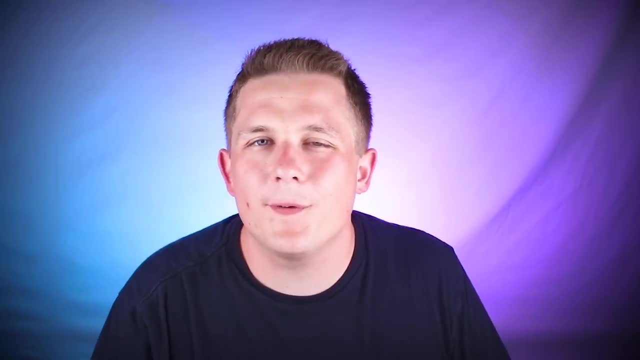 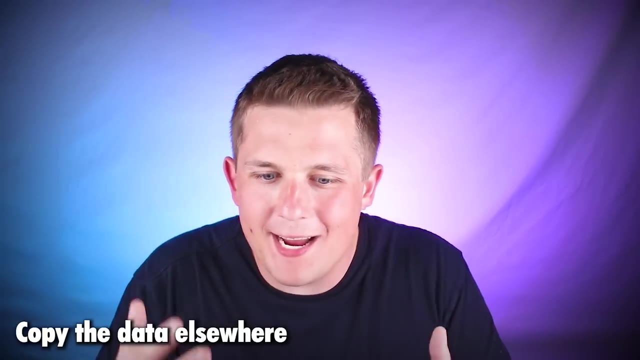 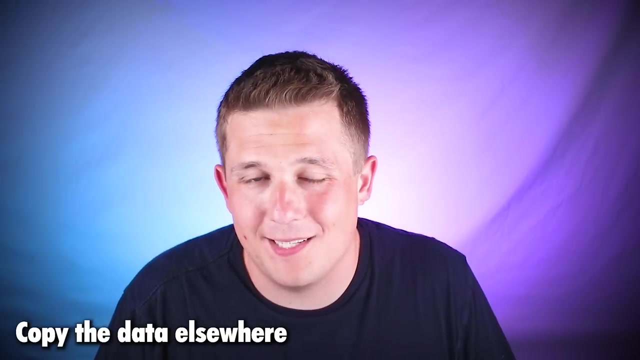 estimator. And finally, the last tip to improve your query performance through refactoring of the data alone is to just create a copy of the data. Sometimes the amount of rewriting you would have to do to get a query to perform better just is too much, or you can't possibly rewrite it to make it perform better without also. 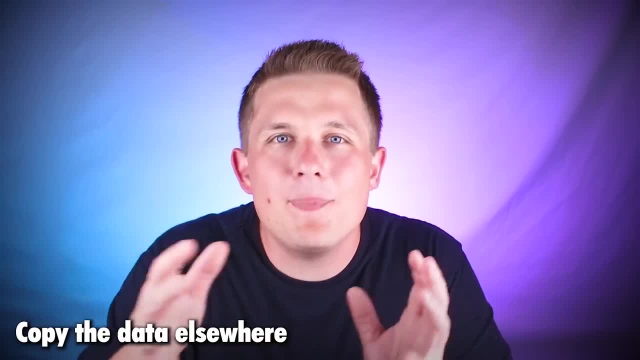 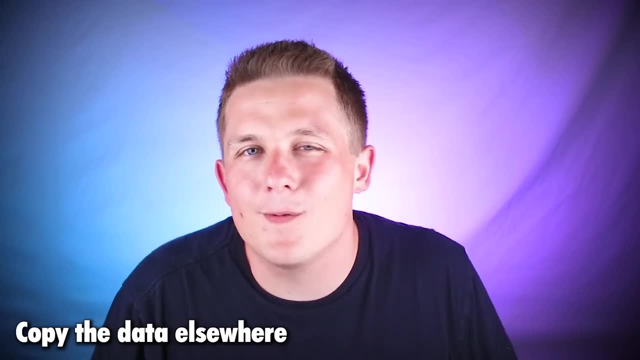 adding indexes and things. So it just makes sense to just make a copy of that data somewhere else and then you have the freedom to create indexes and change settings and have more control over how your queries are executing. So don't ever forget that creating a copy of the data for a different 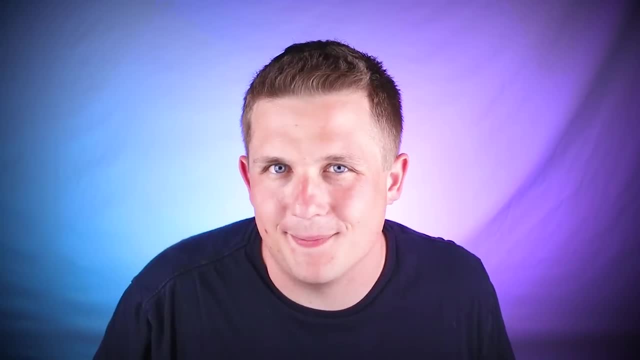 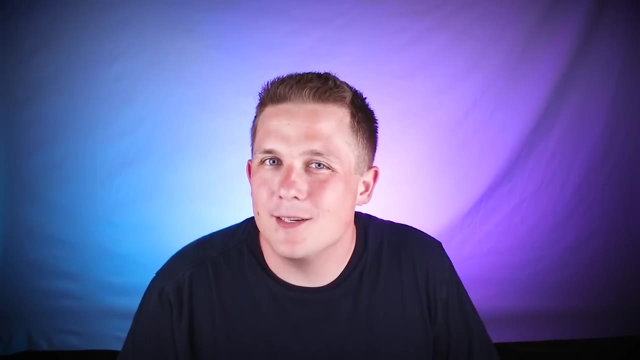 specific purpose for your query is a valid option, And by no means is this list of query rewriting techniques exhaustive. There's numerous amounts of ways you can rewrite a query to improve performance. The key thing to remember is that the SQL Server Query Optimizer is making plans based. 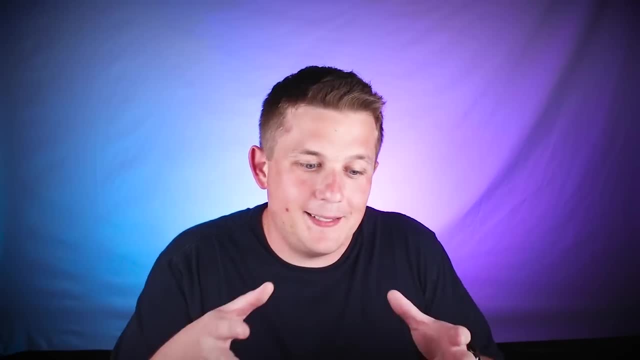 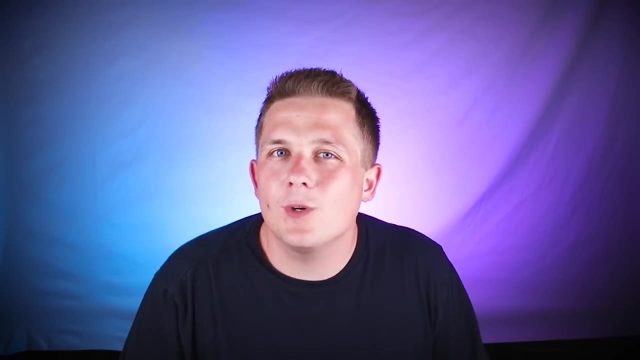 on the best data that it has available, and sometimes either the data that it has available or its assumptions go all out of whack and you get these bad execution plans In those cases if you can't fix the root cause of the problem by modifying indexes.